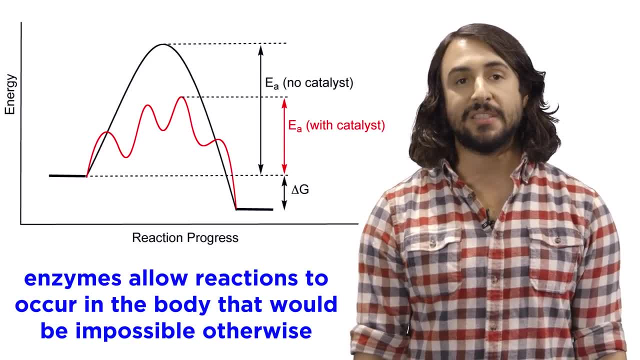 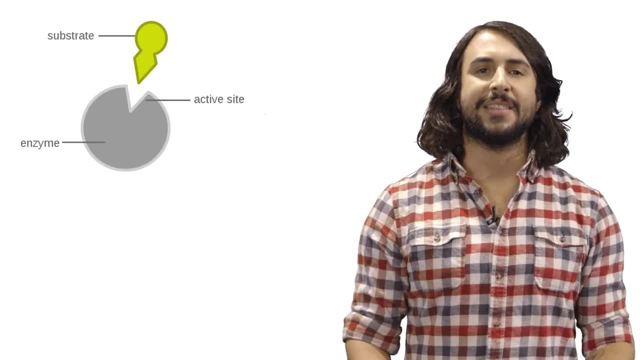 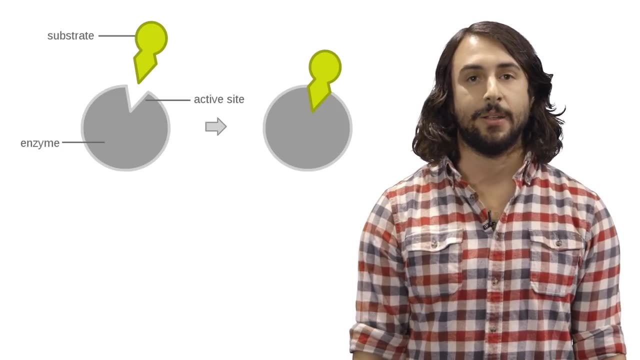 it up to a trillion times more favorable, such that it is feasible to occur on a normal biological time scale. So how do they work? Well, every enzyme has a specific substrate and the enzyme recognizes its substrate with extremely high specificity. So it's kind of like a lock and key where a specific molecule is the key that activates. 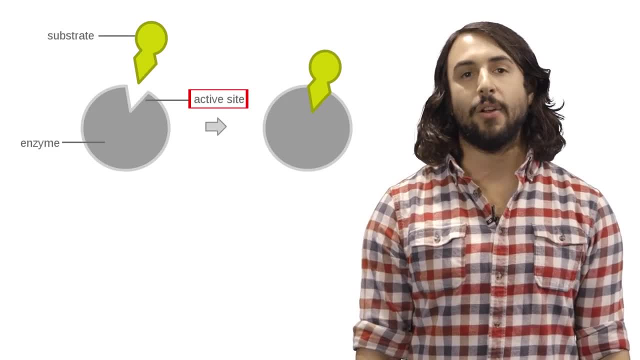 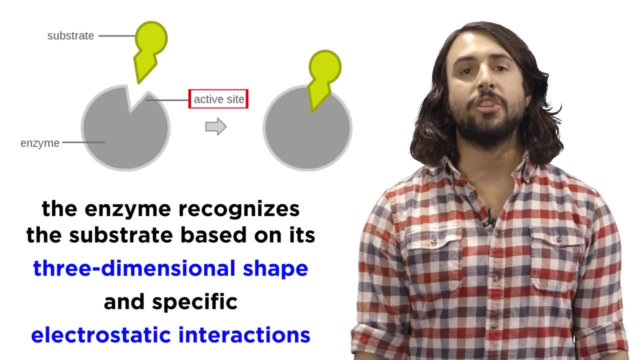 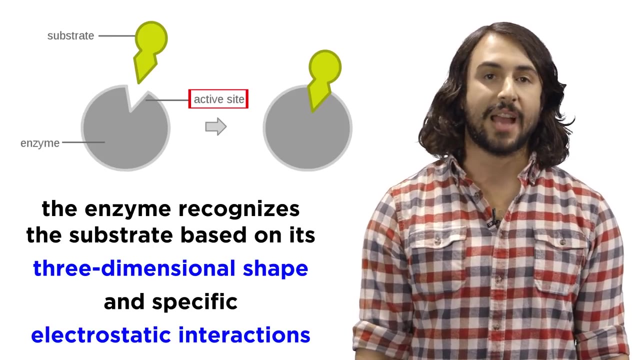 the enzyme's function. There is a specific area on the enzyme that the substrate will bind to, which is called the active site. The substrate will bind to the active site because it has just the right shape and composition to do so, meaning it is the right size, but it also has functional groups that make favorable 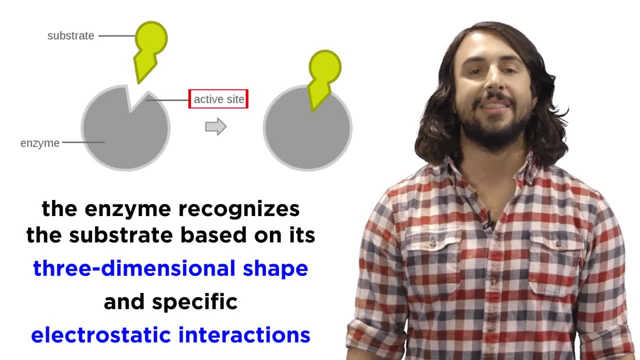 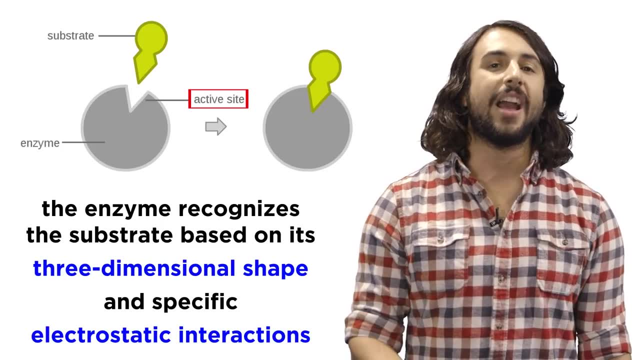 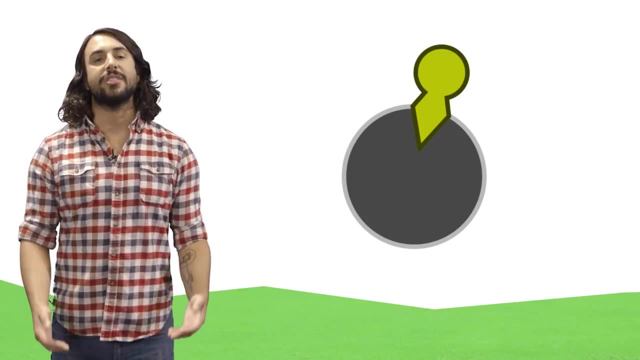 electrostatic interactions with certain key residues in the active site of the enzyme, Whether those are van der Waals interactions, hydrogen bonds or energy bonds. the enzyme will bind to any other interaction of this type. The substrate might fit into the active site as is, or it might cause an induced fit where 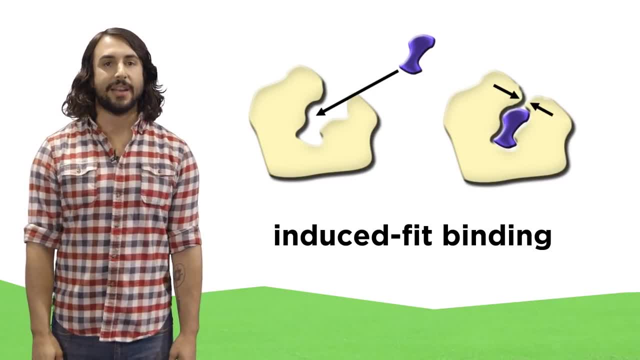 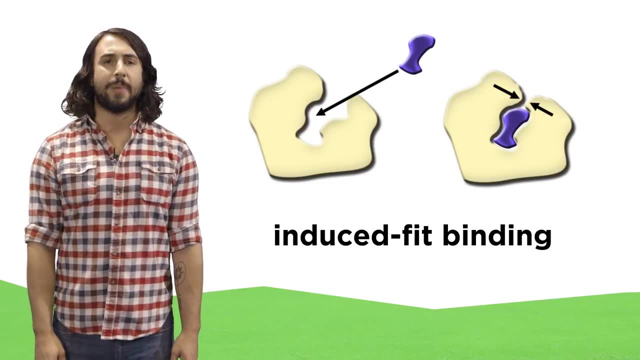 the enzyme changes shape slightly once the substrate is inside, But either way, once the substrate is inside the active site and binding has occurred, a number of things might happen. One possibility is that the enzyme causes the substrate to bend in a particular way. 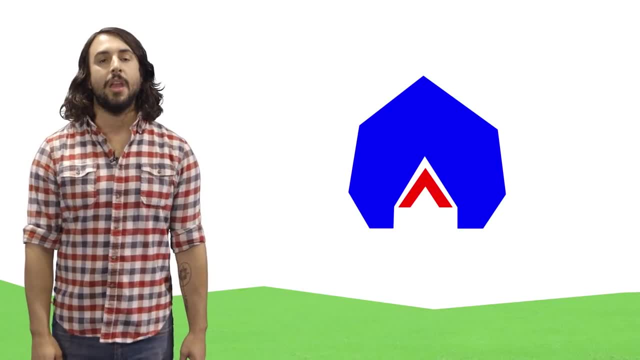 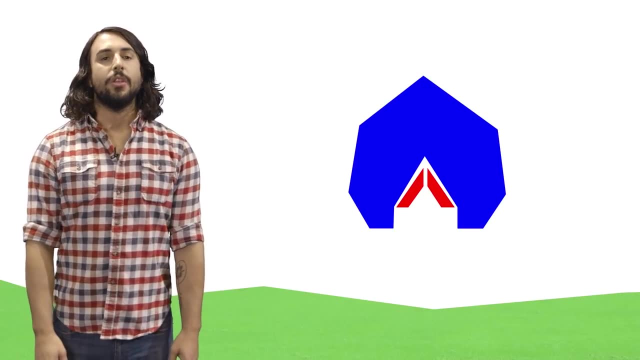 which it will do in order to make certain interactions with the enzyme. And if the enzyme is in the active site, then it will bind to the enzyme And when, in this bent configuration, some of the bonds become weaker and easier to break, This is one way the enzyme qualifies as a catalyst. The molecule would have a hard time breaking apart on its own, but in the conformation induced by the enzyme, the activation barrier associated with the reaction is much smaller. So many enzymes have the task of breaking down large molecules like the ones we eat. 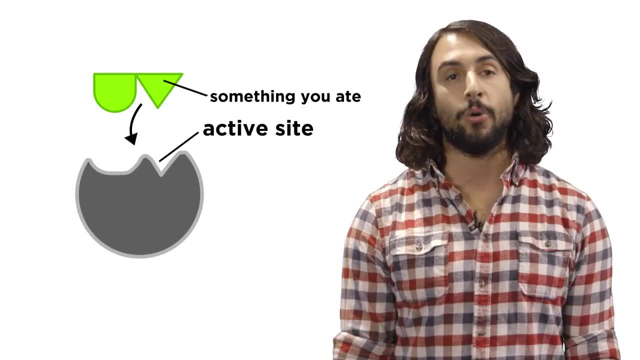 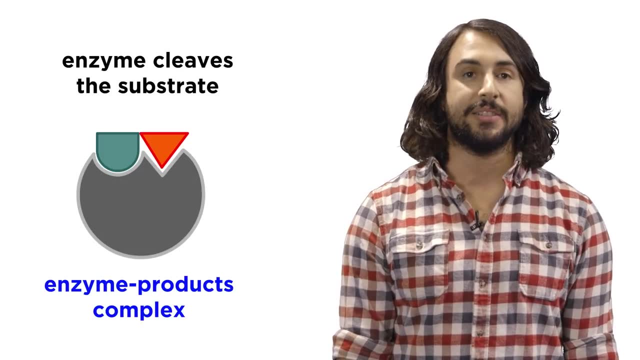 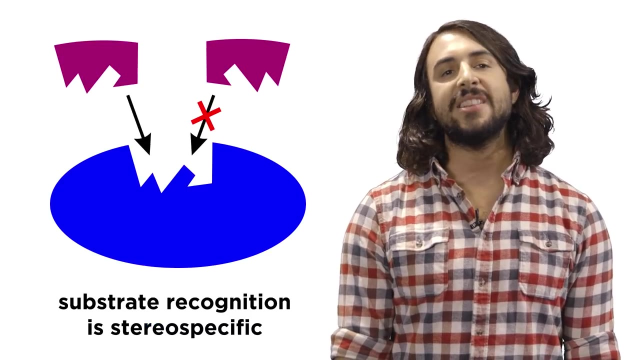 to form the tiny components that we can use to break down large molecules. Once the enzyme catalyzes the reaction, the reaction proceeds, the altered substrate leaves and the enzyme can then go and catalyze another reaction. Enzymatic activity is always stereospecific, meaning that if a substrate can exist as two, 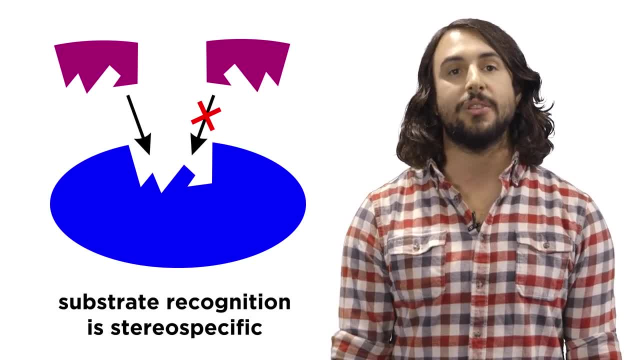 mirror images. only one of those forms will fit into the active site of the enzyme. Most enzymes have names that end in a triangle. Most enzymes have names that end in a triangle, which we'll discuss in a little bit. If the substrate in an activate formation is active, then it can be used to bind to the active site of the enzyme. 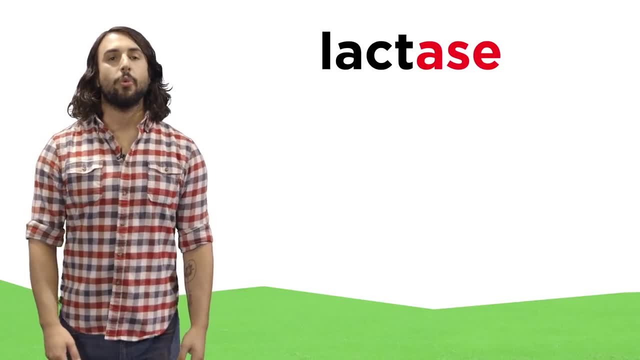 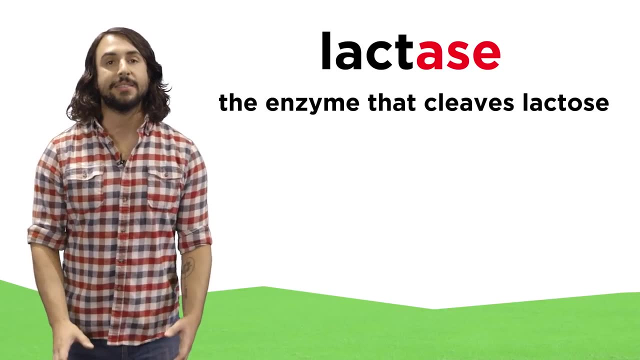 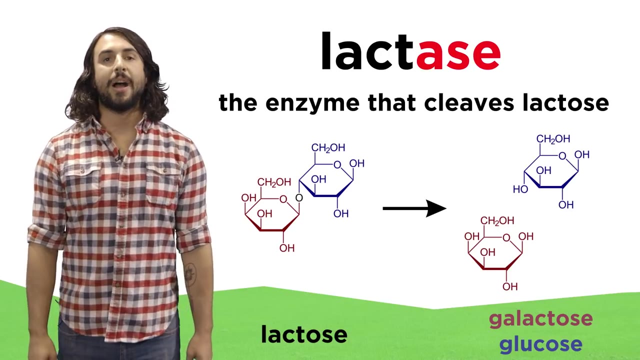 ACE, so you'll know an enzyme when you hear one. The rest of the name usually has to do with what the enzyme operates on. For example, the enzyme lactase breaks down lactose, the sugar found in milk, into two smaller sugars. We will learn. 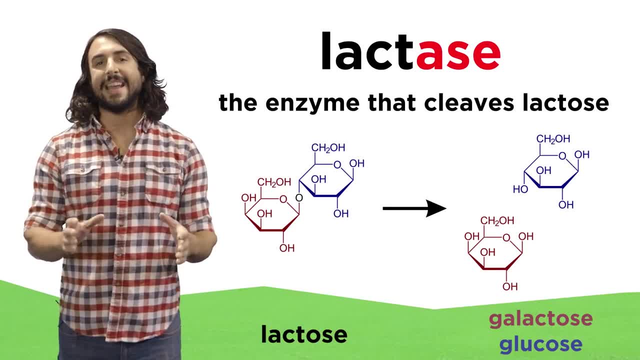 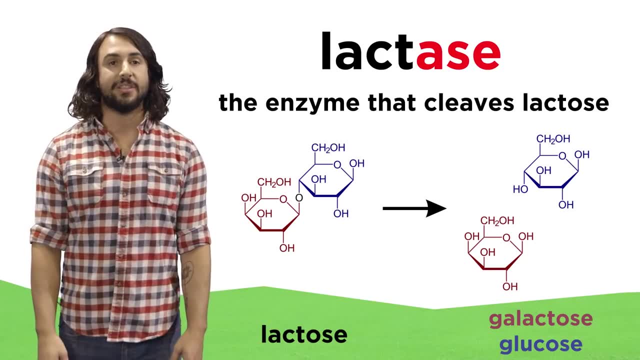 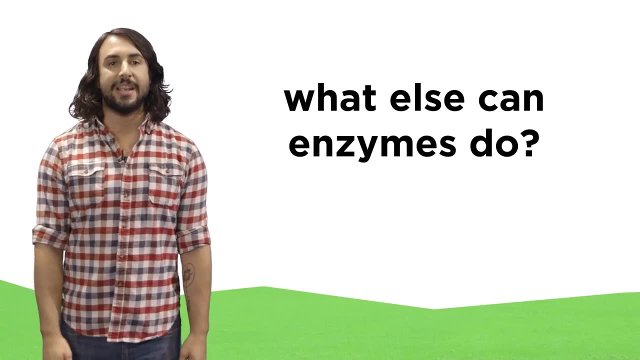 about these types of molecules. next, It is a deficiency in lactase that causes lactose intolerance in some people, because without enough of this enzyme it is very difficult to digest lactose, as nothing is present to break it down once ingested. But breaking down molecules into pieces isn't the only thing that 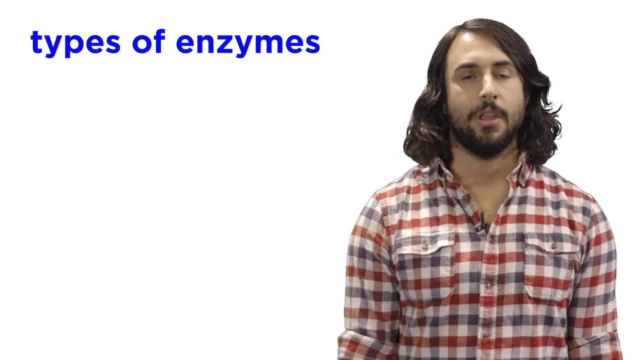 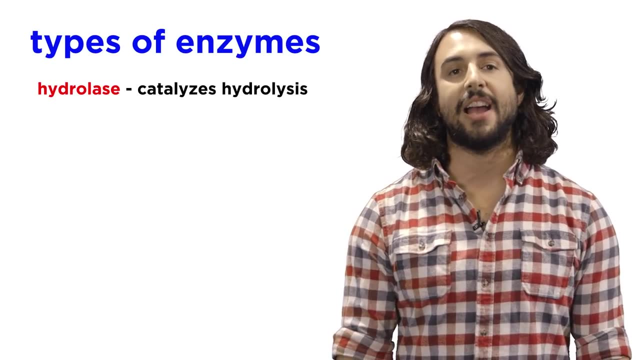 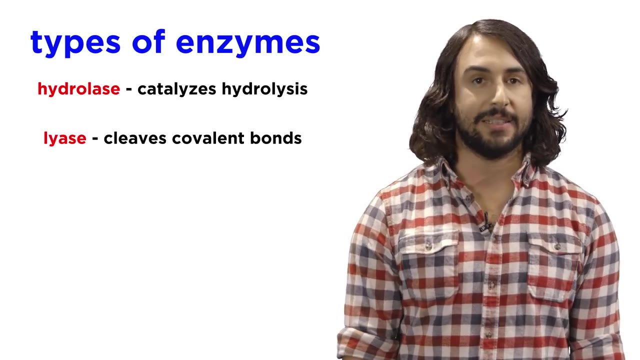 enzymes can do. Let's look at the categories. We already mentioned enzymes that break down molecules, and those could be a hydrolase, which catalyze the hydrolysis of a chemical bond, which effectively separates a molecule into two pieces, or a lyase, which also cleaves covalent. 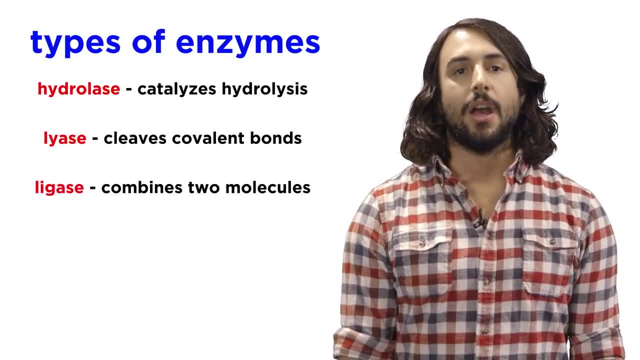 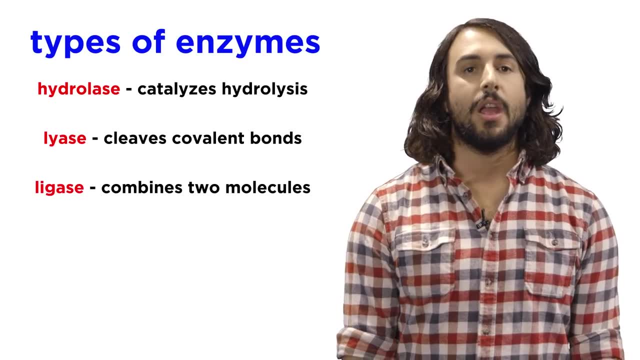 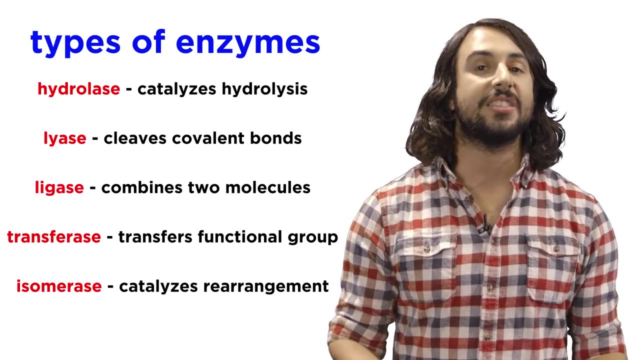 bonds, but by means other than hydrolysis, An enzyme with the opposite function. a ligase is an enzyme that joins two molecules together. a transferase is an enzyme that transfers a functional group from one molecule to another. an isomerase catalyzes a spatial rearrangement of the 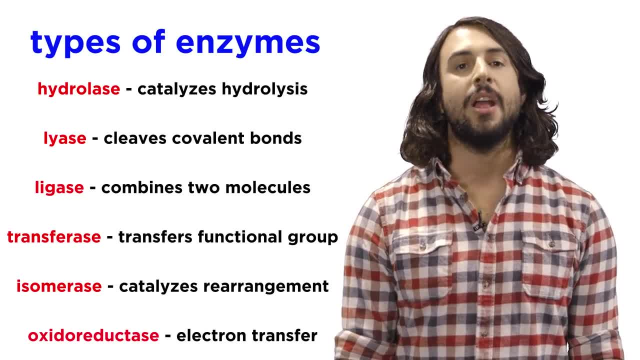 substrate, and an oxidoreductase is an enzyme that transfers electrons from one molecule to another. Sometimes, when an enzyme operates on its substrate, itこんな versteres neeها, не думаю untuk nenhum modul eigen rumens. 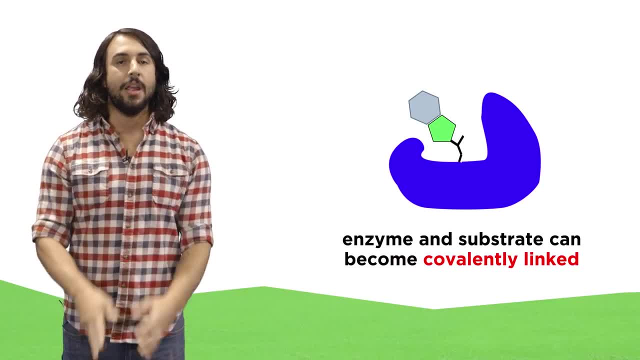 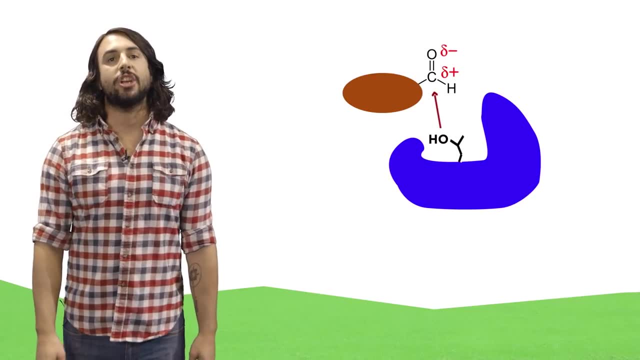 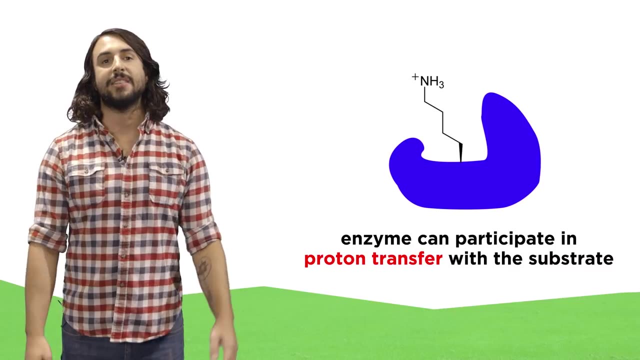 they will temporarily become covalently linked. this can happen if a residue in the active site has a nucleophilic group, like the hydroxyl group on serine, which can react with an electron deficient atom in the substrate, kind of like an SN2 reaction. sometimes an enzyme simply does acid-base catalysis, meaning it. 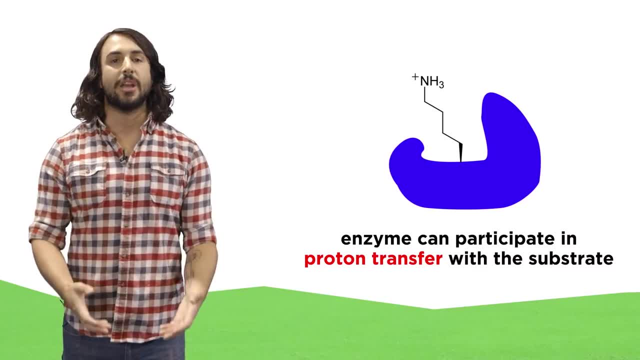 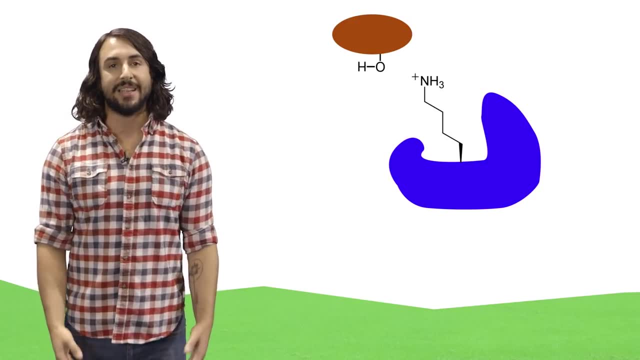 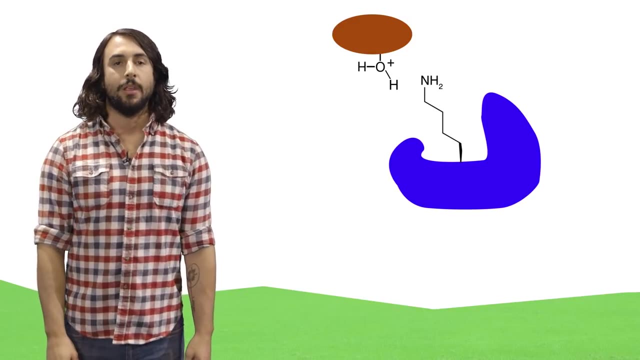 either donates a proton or accepts a proton from some functional group on the substrate to make it more reactive. an example of this is when a residue in the active site is acidic, like lysine, which, if protonated at the amino group, can donate this additional proton. sometimes, in order to function, an enzyme requires. 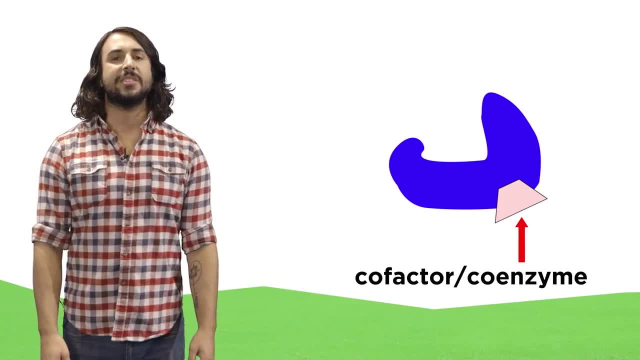 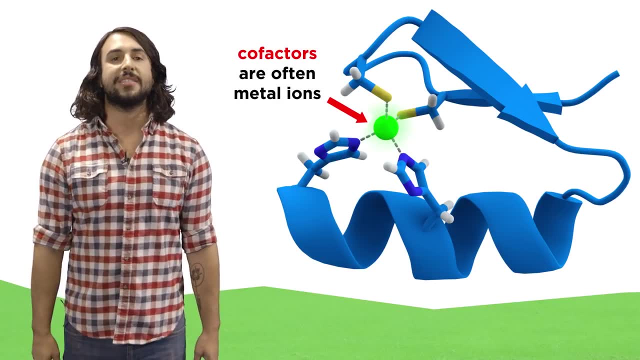 certain cofactors or coenzymes. this is some other thing that must also bind to the enzyme before it can operate on the substrate. cofactors are things like metal ions, whereas coenzymes are actual organic molecules, molecules like vitamins. that's why we